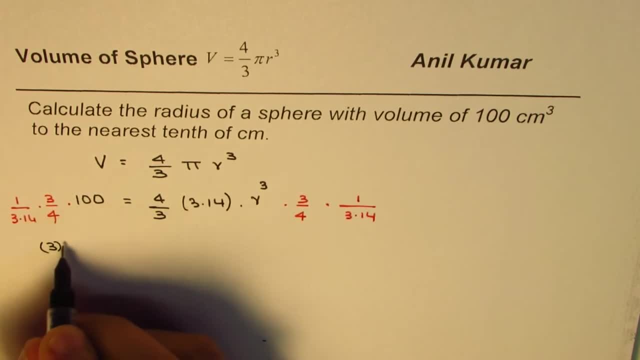 here is 3 times 100 divided by 3.14.. All these brackets means product right Equals to r cube, Is it okay? So we get the value of r cube cube root? i mean, to get r we have to find cube root of this. so that is the reverse calculation. 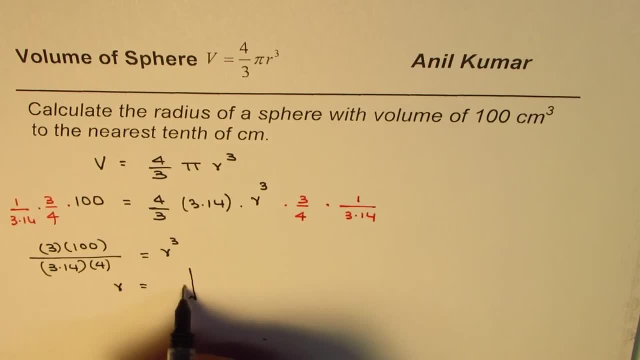 right, so r will be cube root. that is how we write and we can multiply these things, so i'll do it at the end. i'm using multiplication sign now. you could write them in brackets also: 3.14 times 4, right? since different students use different kind of techniques, i've mixed them up. 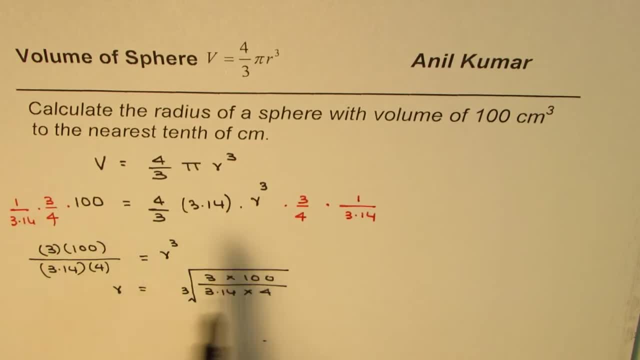 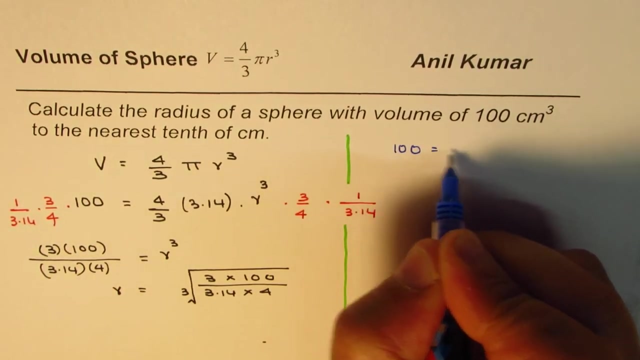 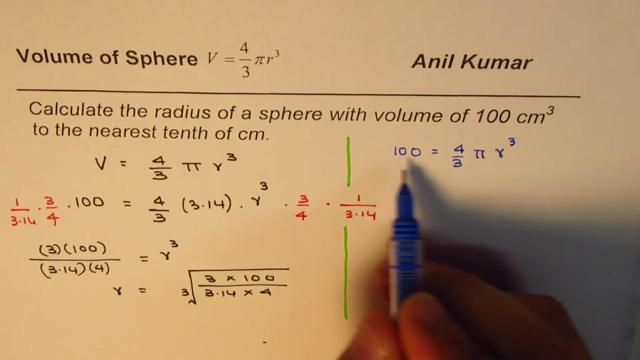 correct. so that is what we did. we did kind of reverse calculation and we can use calculator to find this answer right now. some of you could do direct. for example, we had this: let's redo: we have 100 equals to 4 by 3 pi r cube. so to find r, we'll do, we'll cross multiply, so we'll do three times. 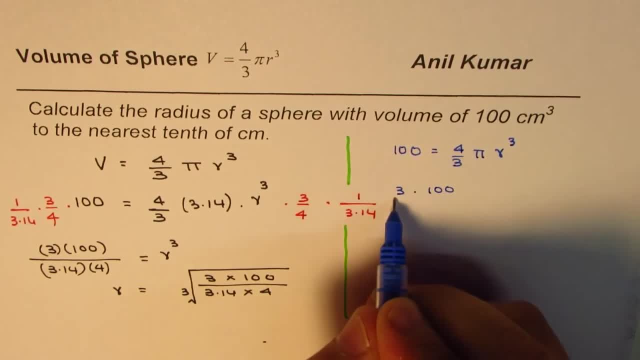 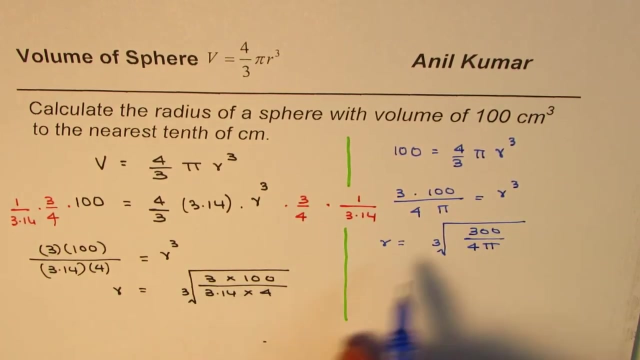 100 right. divide by 4, okay, divide by pi- equals to r cube, and then we can calculate r by finding cube root of this. so r equals to cube root of. let's multiply 300 over 4 pi, is it okay? so this is another way, but the same thing, do you see? but i'm using pi here, not 3.14, which is kind of a. 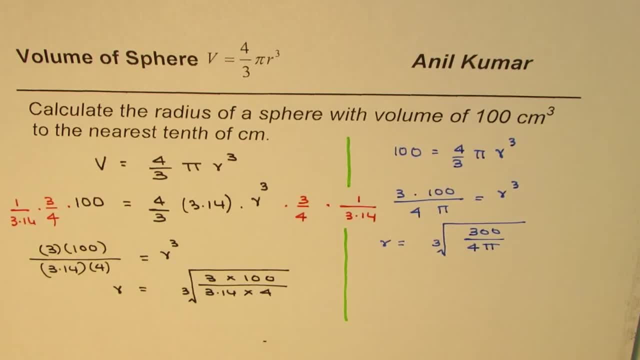 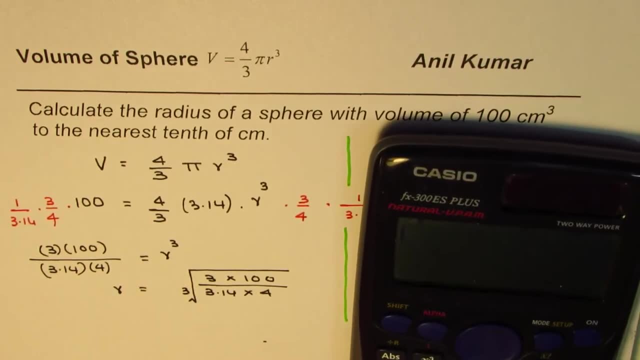 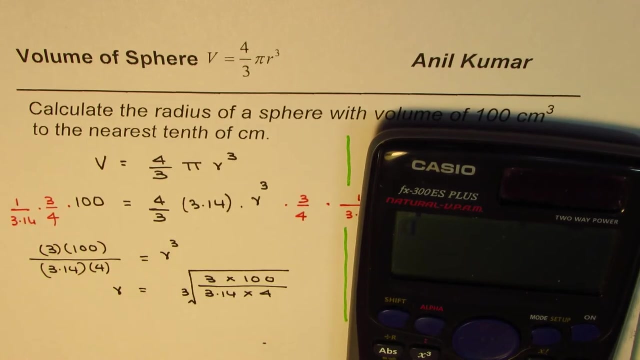 proxy, but close enough anyway. let's use calculator now to find the cube root of what we have here. so let's put all this within within brackets. so we have bracket three times hundred. three times hundred divided by, within brackets, four times 3.14. bracket close. 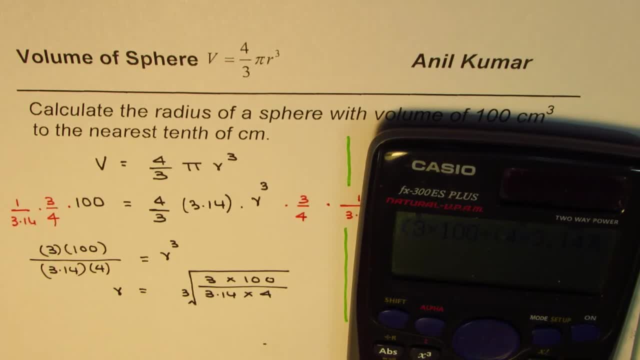 now. so we we can divide this now, since- look here, we have one bracket here, so 300 divided by both of them- bracket close. we have to use another bracket to close for the first one. okay, and the power is cube root. we could write this power as: 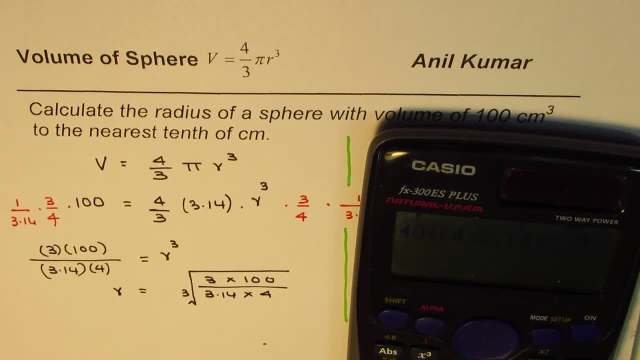 one over three, right, so we could write this as power of one divided by three. power, correct. and now 10ず皆, and now we can say: and now we can say equal to, to get the answer. so the answer for this is 2.879 centimeters, right, so units of centimeters. 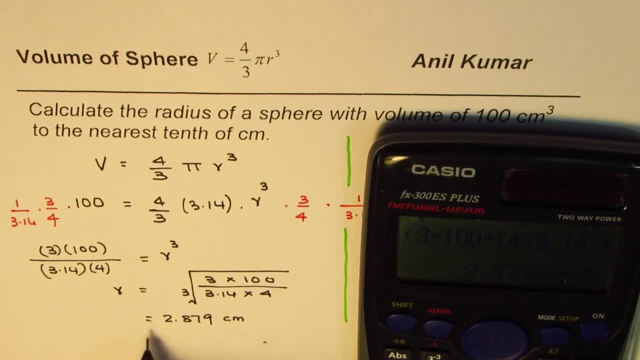 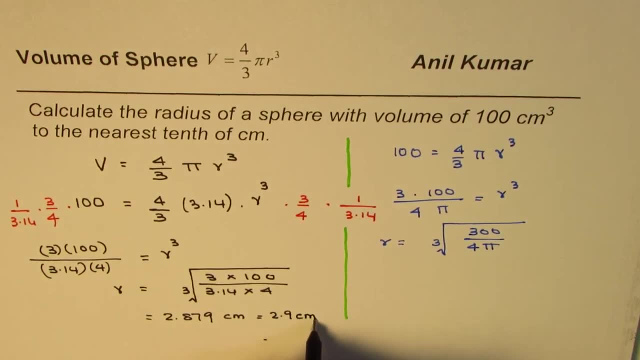 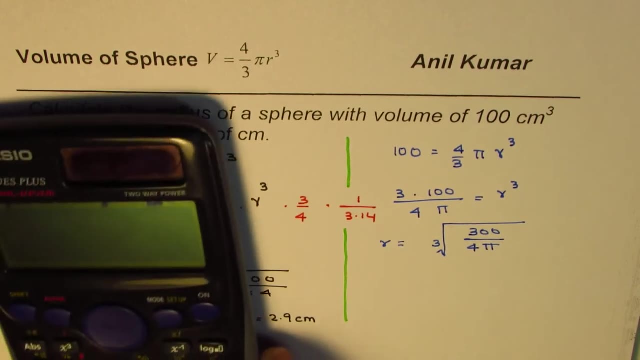 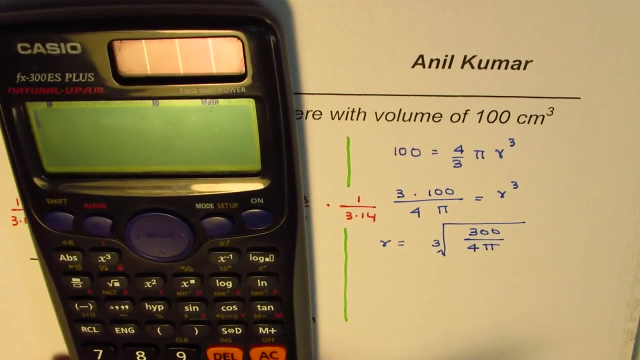 which you could round to one decimal place as equal to 2.9 centimeter. good, so that is how you would calculate this. okay, let's do the next one also, which is cube root of. we'll use pi this time, right? so so we are using cube root in the calculator. 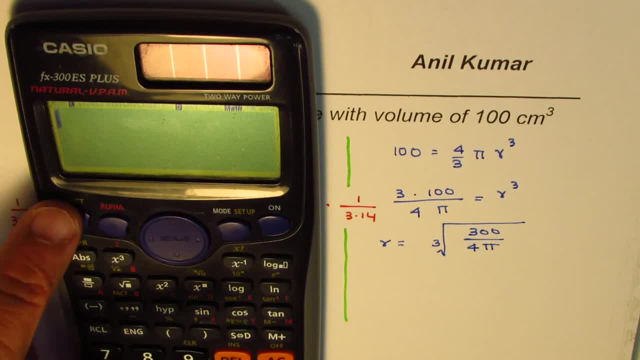 you may have cube root function correct so we can say shift cube root so that gives you cube root directly. we do not do exponent 1 over 3 as we did last time, so that's kind of an alternate way so we have within the cube root. we could do fractions also, but many calculators do not have. 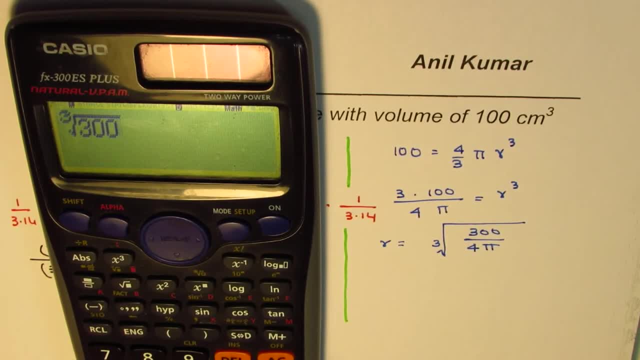 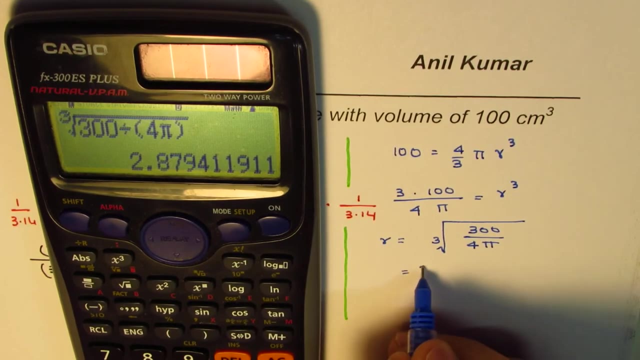 that, so i'm not using this. okay, 300 divided by uh, let me put in brackets 4 pi, so 4 shift pi, so you get 4 pi. good, now let's calculate this value. it is equal to 2.879, right? so it could be approximately as: 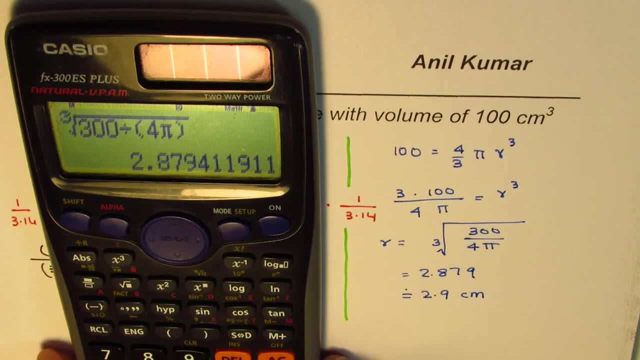 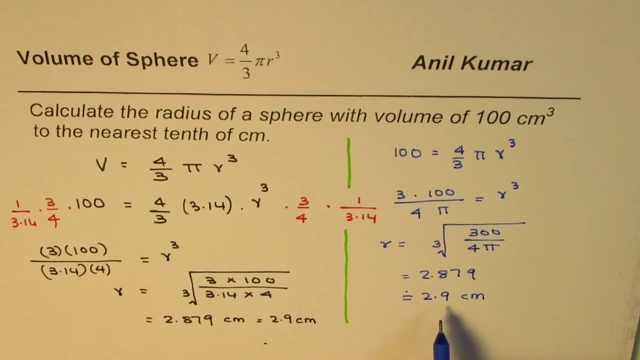 2.9 centimeters. perfect, so you get exactly the same answer in this particular case. so you could always approximate pi to 3.14 when you're finding the radius okay. so our answer is: radius is equal to 2.9 centimeter, correct? now you could do reverse. i mean we've done the reverse.